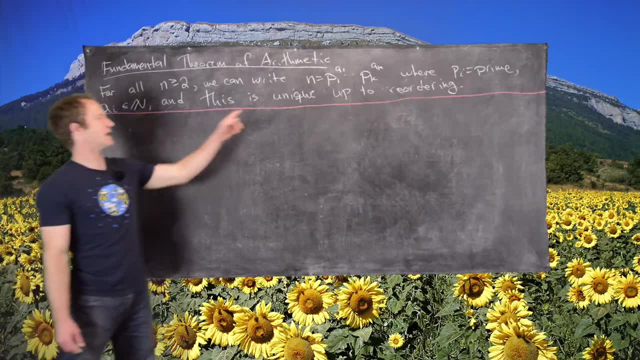 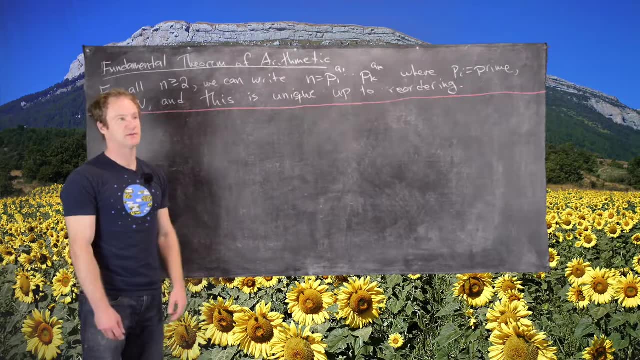 The AIs are natural numbers and this product is unique up to reordering. So, for example, 6 can be written as 2 times 3 or 3 times 2, but we'll consider those as the same representation in terms of primes, because it's just a simple reordering. 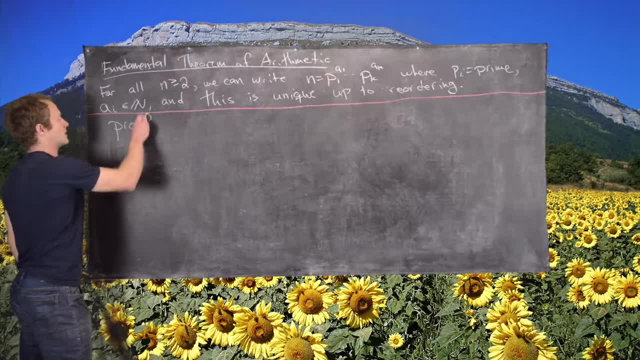 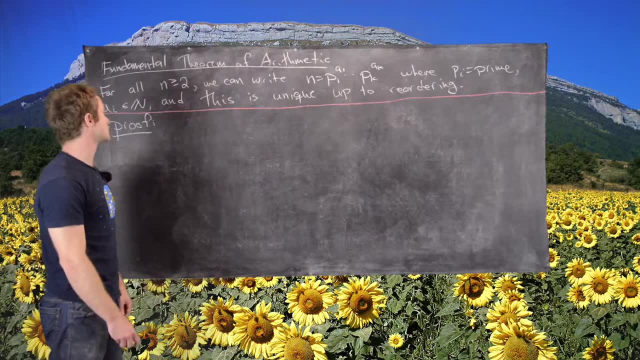 Okay, great. So now we're ready for this proof. So we have two things to do. First, we need to know the number of times that the product P1 to the Ak is equal to. Second, we need to prove that for all natural numbers bigger than 2, there exists a representation as a product of power of primes. 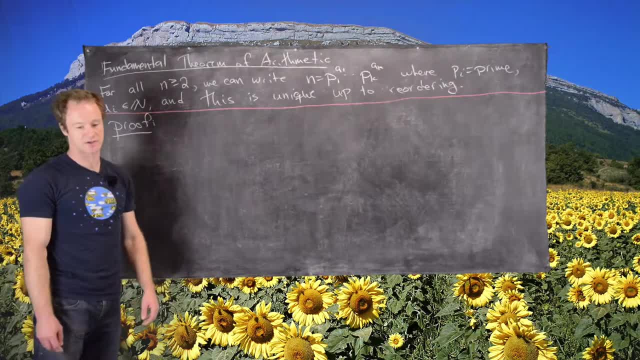 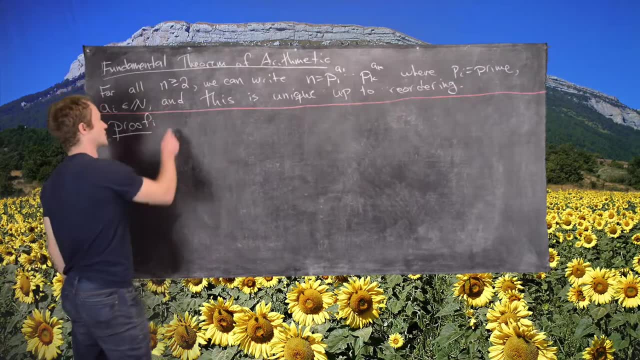 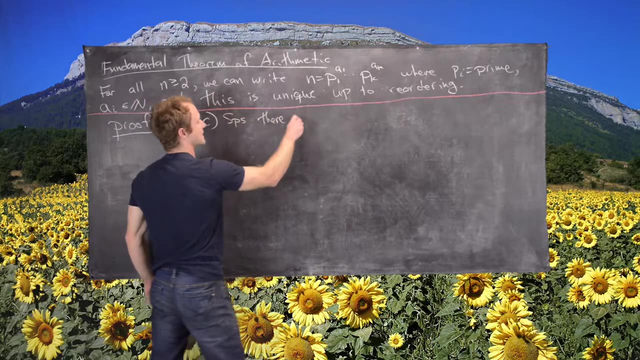 And next we need to show that that representation is unique, up to reordering. And so what we'll do first is show that there is a representation, So we'll do that by way of contradiction. So, by way of contradiction, suppose there is a natural number. 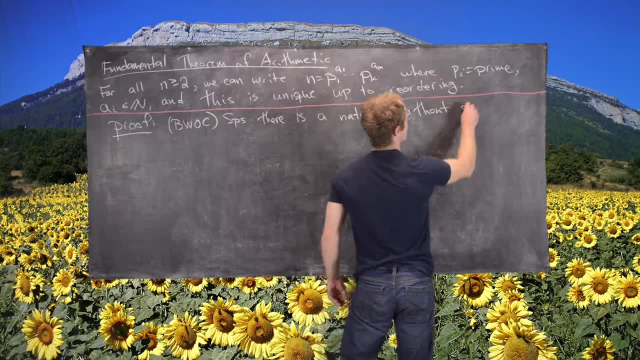 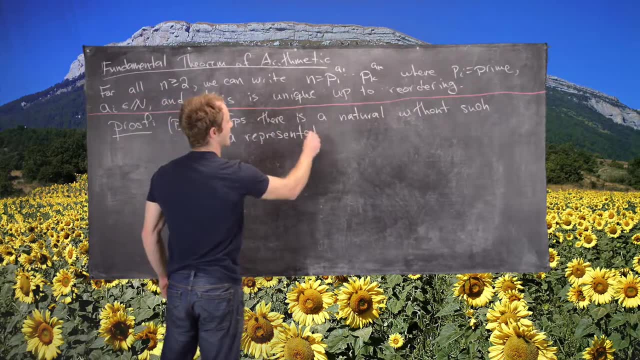 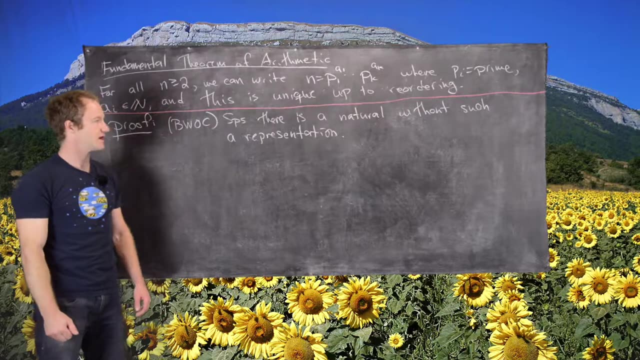 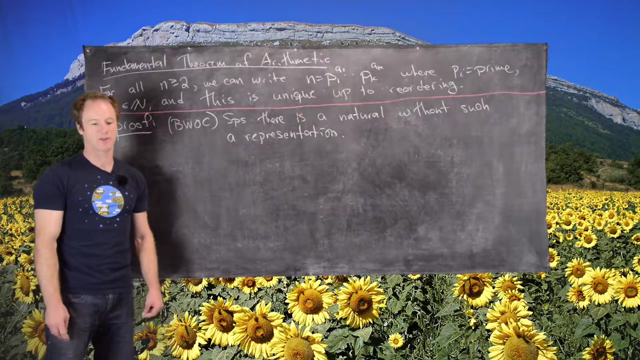 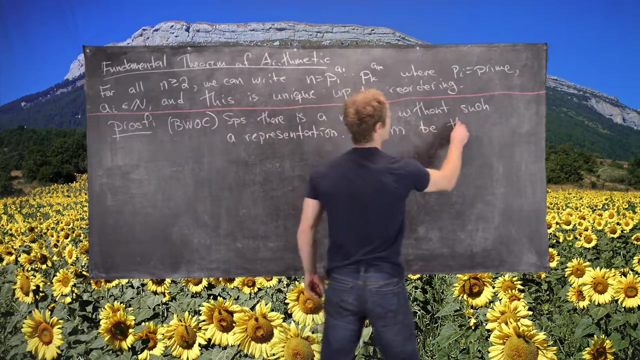 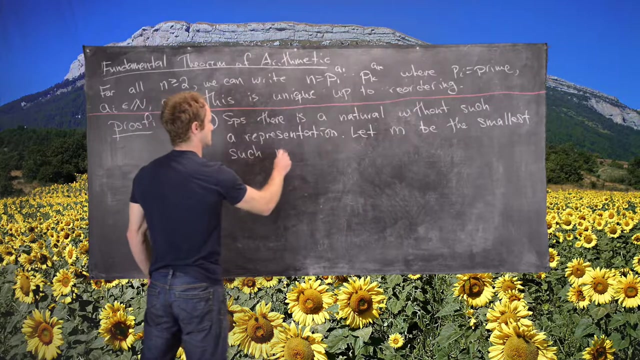 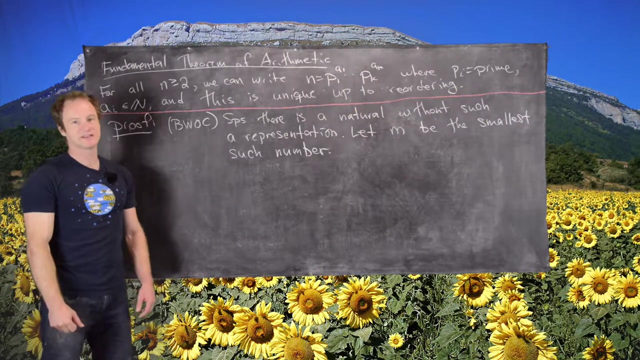 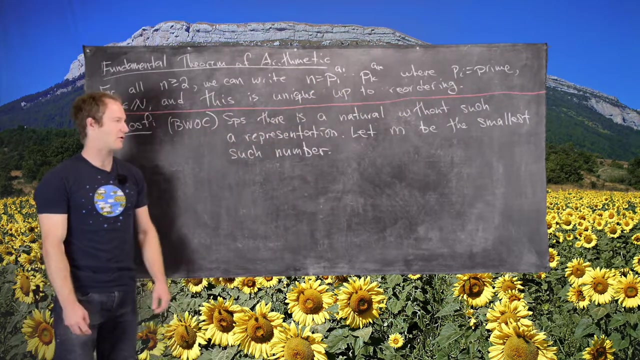 So if there is a natural number without such a representation, there is a smallest natural number without such a representation. So that's what we'll do. So let's let M be the smallest such number. Good, So just to reiterate, M is the smallest natural number with which you cannot factor it into a product of power of primes. 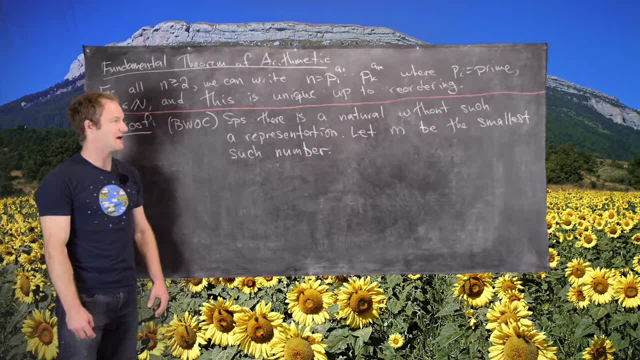 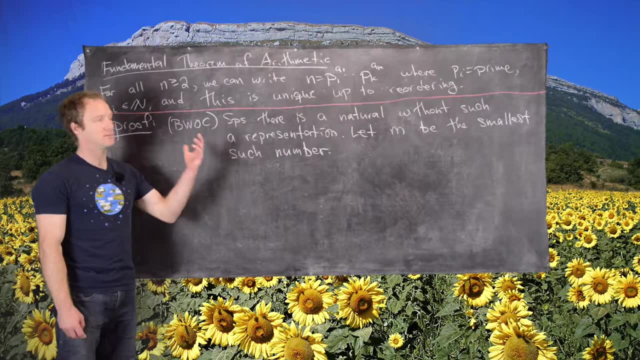 Good. So now what we'll notice is that M must be composite. So if M is prime, then M equals P to the 1 power, But obviously P to the 1st power is in this form. So M must be composite. 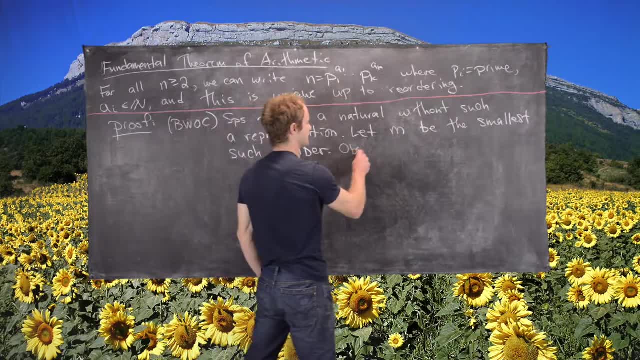 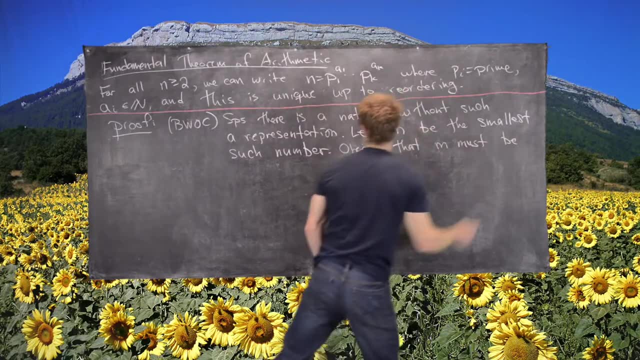 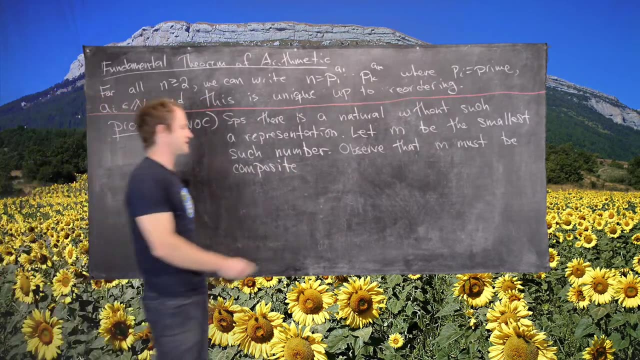 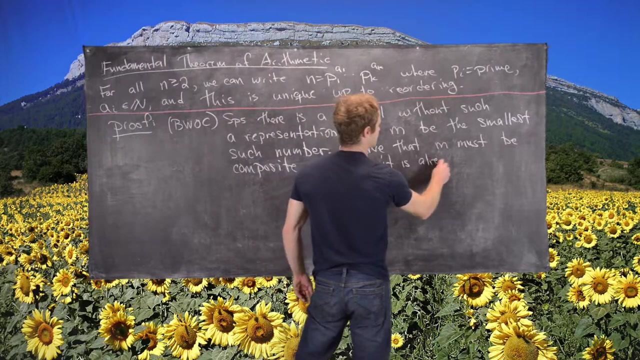 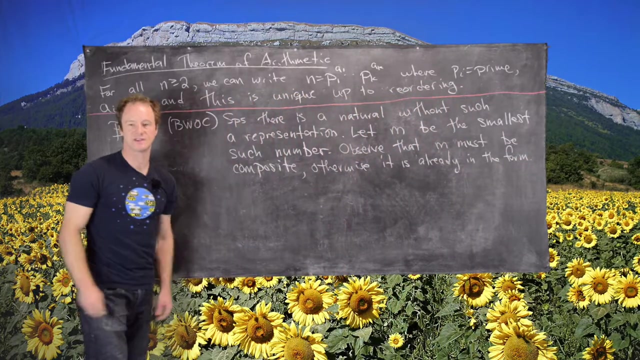 So we'll just write that here. So observe that M must be composite So, and then we'll just like briefly write, otherwise it is already in the form, And by the form I mean the representation of a product, of powers, of primes. 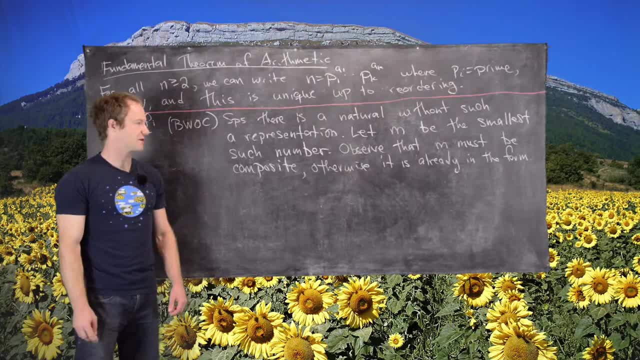 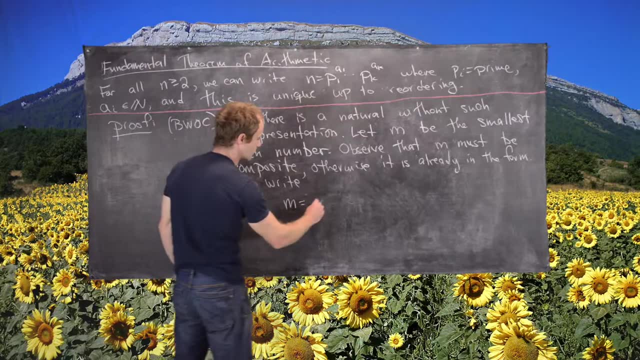 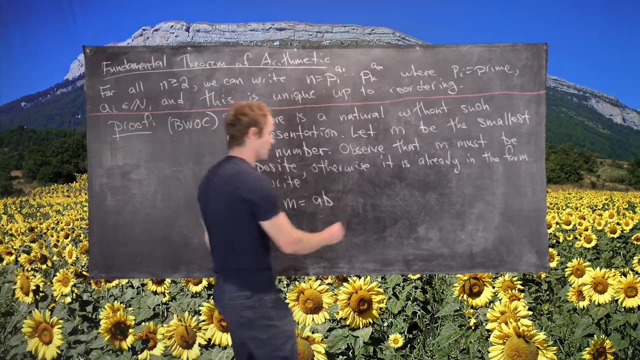 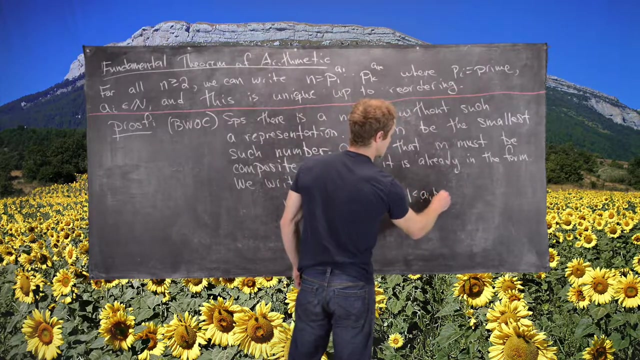 Okay, good, So since M is composite, we can write. So we write the following: M equals A times B. So recall: a composite number is a number that can be factored where A and B are between 1 and M, not including 1 and not including M. 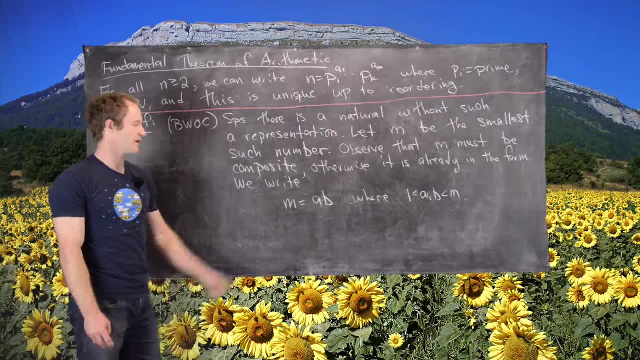 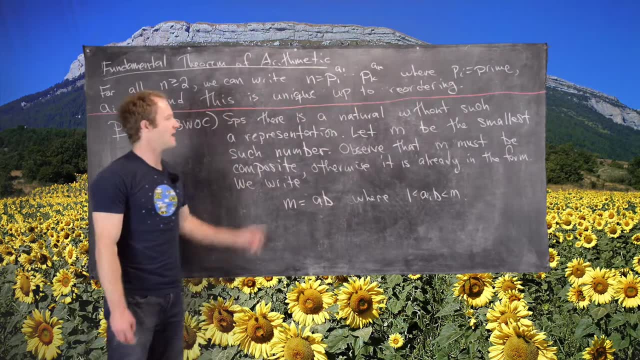 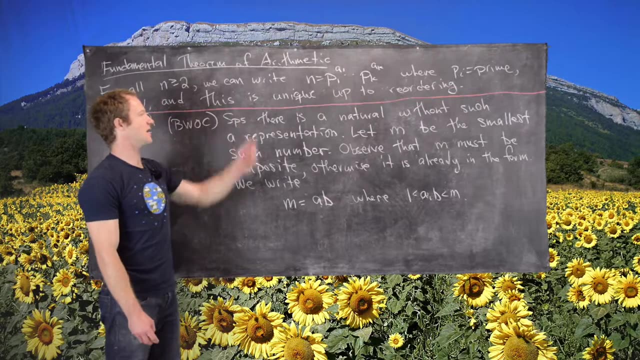 So that's the definition of a number being composite. Okay, great. So now, since A and B are both smaller than M, and M is the smallest such number, that means A and B are representable as a product of power of primes. 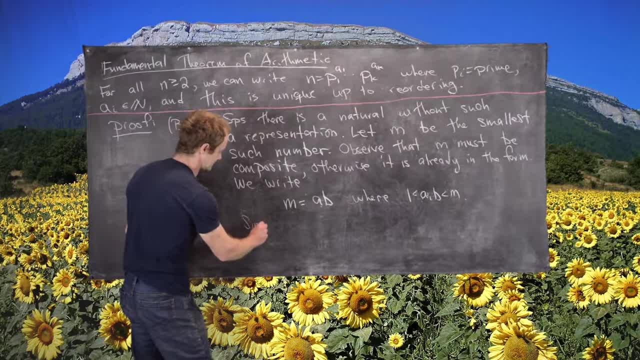 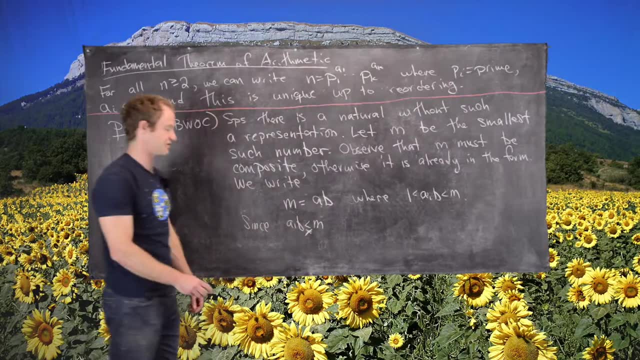 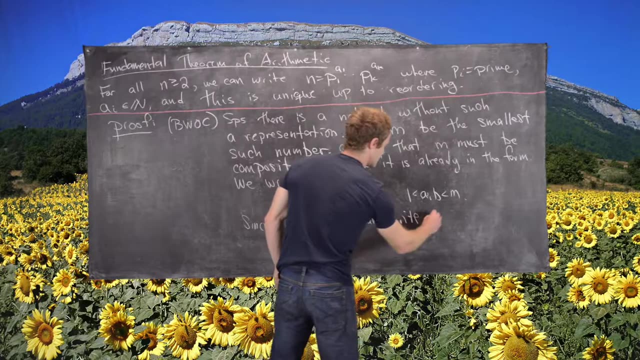 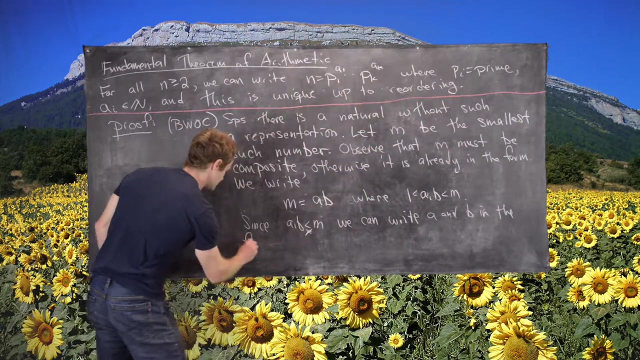 So let's notice that. So since A and B are smaller than M and not equal to M, so let's like put a not equals there. just to point that out. So we can write A and B in the form given. 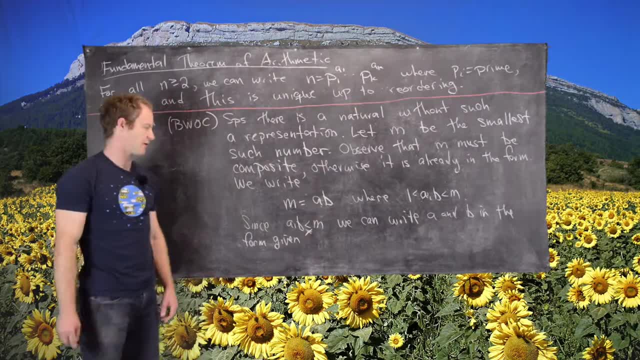 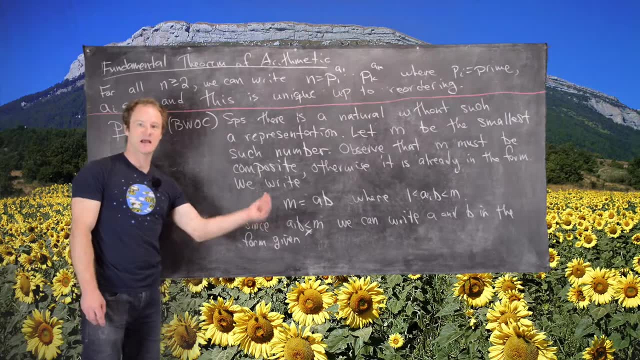 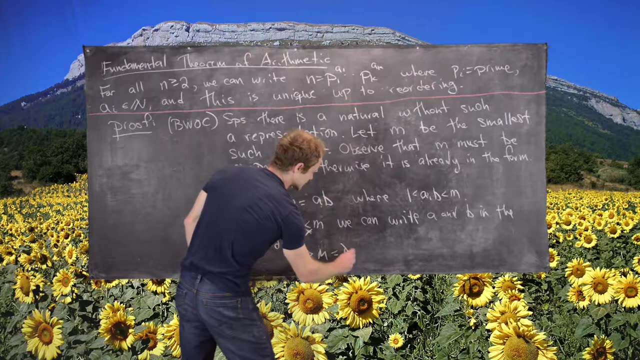 So what I mean by that is the product of power of primes. But if A and B can be written as the product of powers of primes, then A times B can, and thus M can. So M equals, And I'll just jump right to the end. 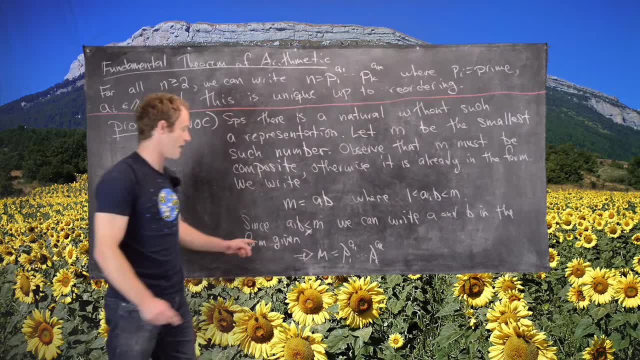 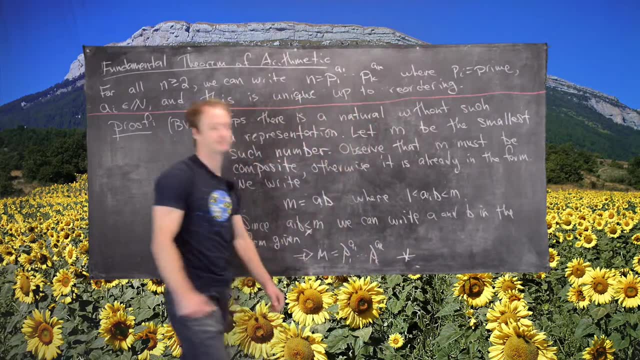 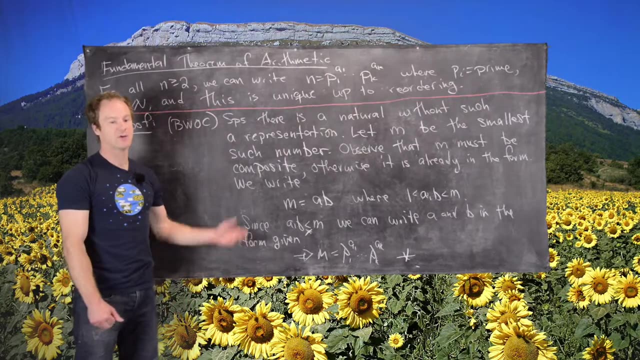 P, K, A, K, Where those numbers are built from the representation of A and B. And this is our contradiction. Okay, so good. We have proven that every number can be written as the product of power of primes. Now we want to show that this way of writing a number 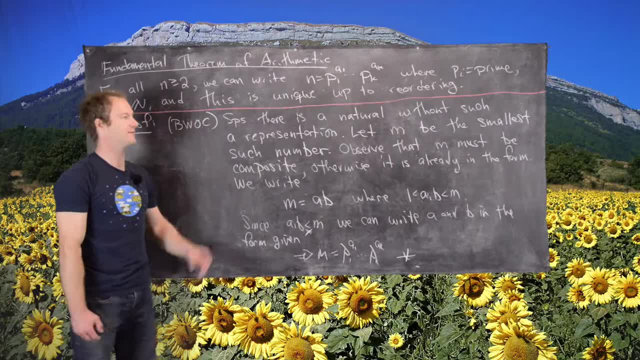 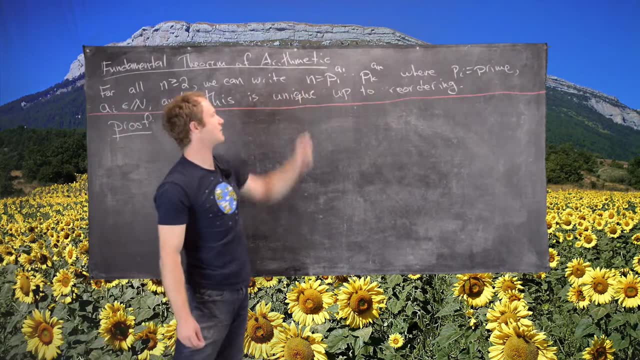 or this representation of a number is unique up to reordering. So I'll clean up the board and then we'll do that. Okay, good. So just previously we proved that every natural number can be written as a product of powers of primes. 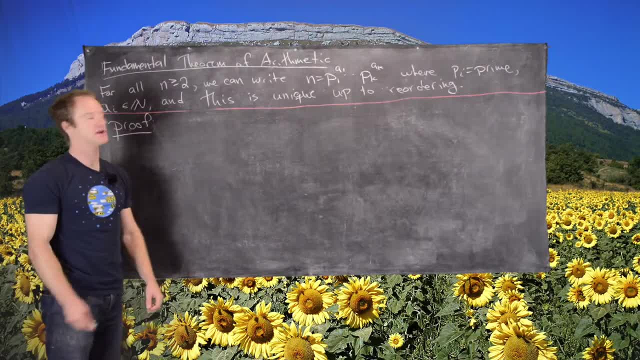 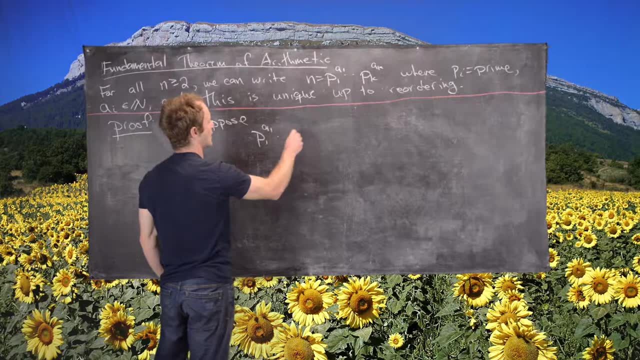 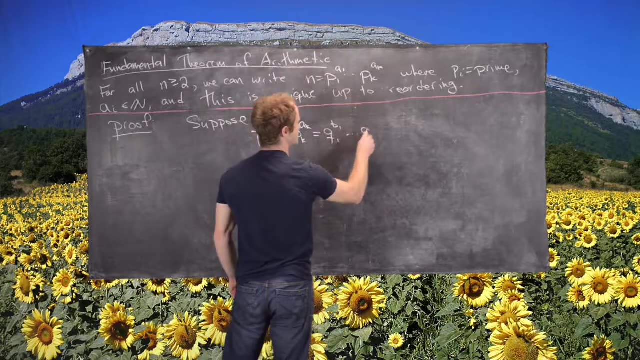 And now we want to show that this representation is unique. So let's suppose that P1 to the A1 all the way up to P? K to the A K equals Q1 to the B1 all the way up to Q? L to the B? L. 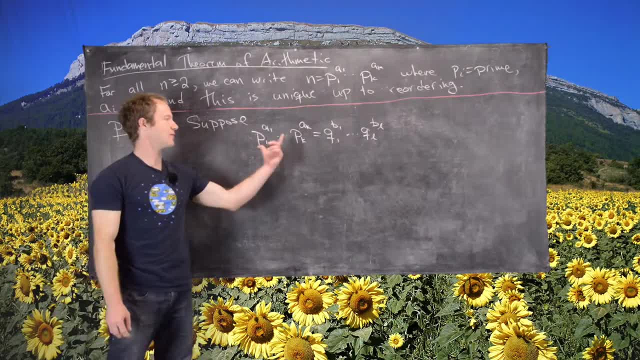 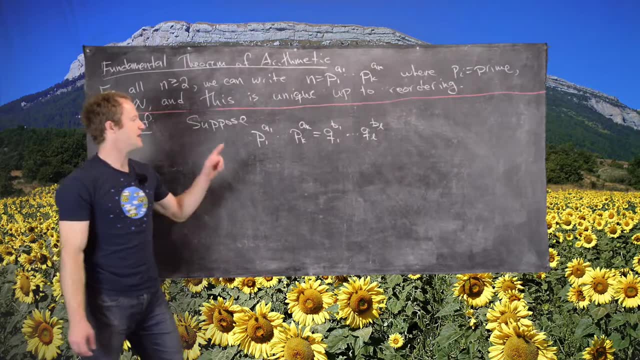 So, in other words, we have the same number represented as two products of primes, And so we have a couple of things to do here. We need to show that K is equal to L, So we have the same number of primes here. 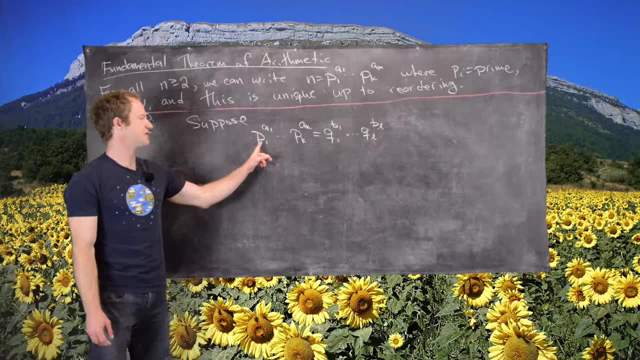 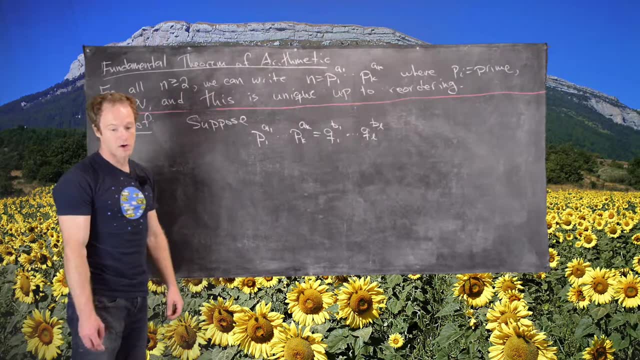 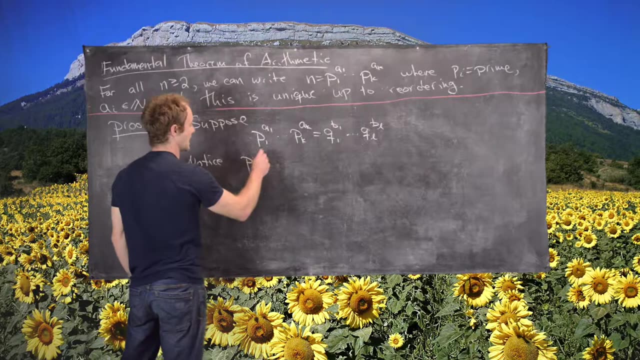 And we also need to show that each of these P I over here is one of these Q I and vice versa. Okay, good, So now let's notice this. So notice that P I divides the left-hand side of this equation. 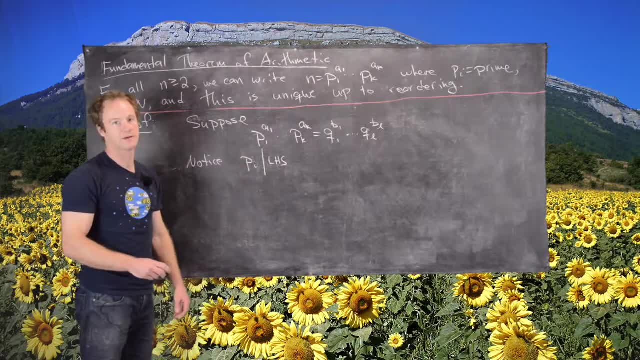 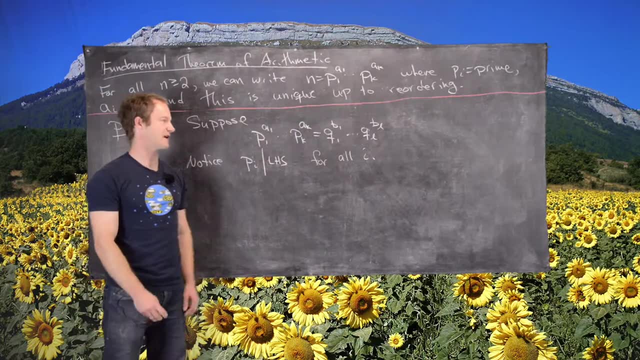 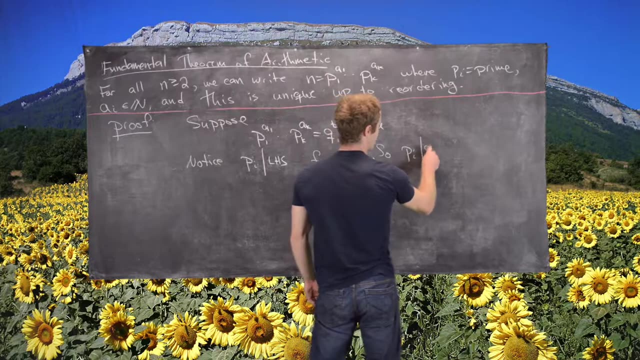 All right. so, and that's true for all I. So let's write that: So for all I. And that's obvious because this is built out of the P I. So that means P I divides the right-hand side. but I'll write that out. 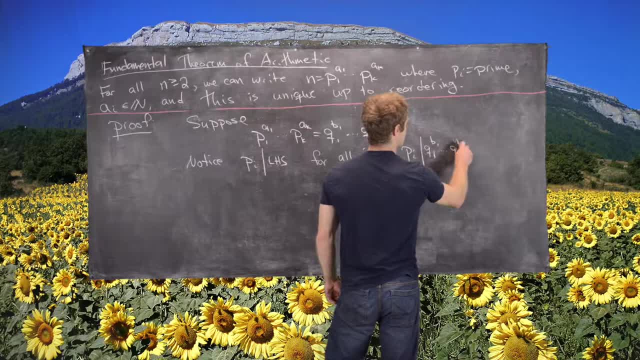 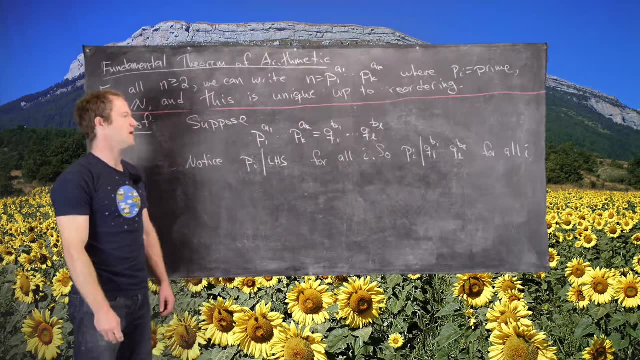 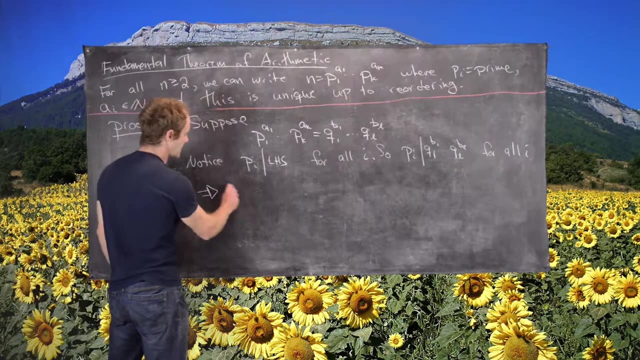 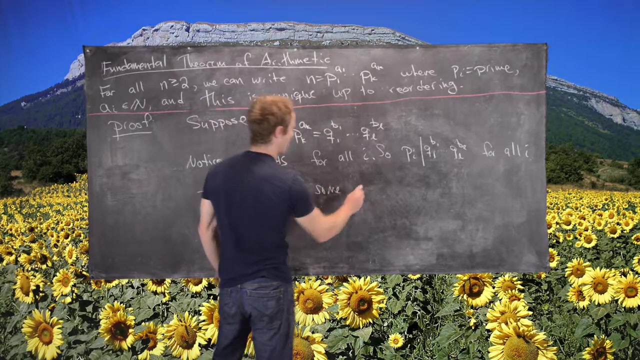 B1 up to Q L to the B L for all I Good. So now what that means by a previous lemma. So that tells us that P I divides Q J. Actually, let's write that as Q R to the B? R for some R. 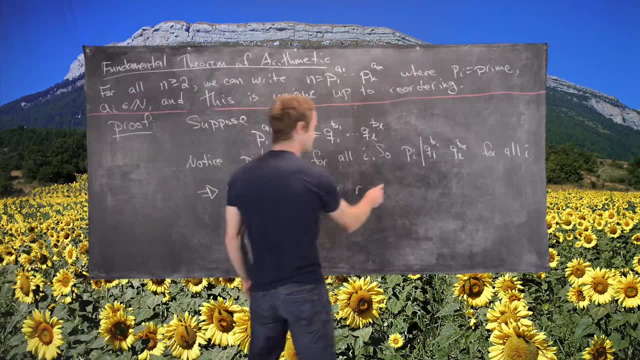 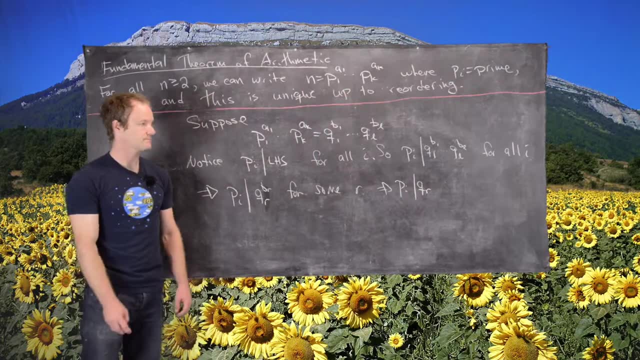 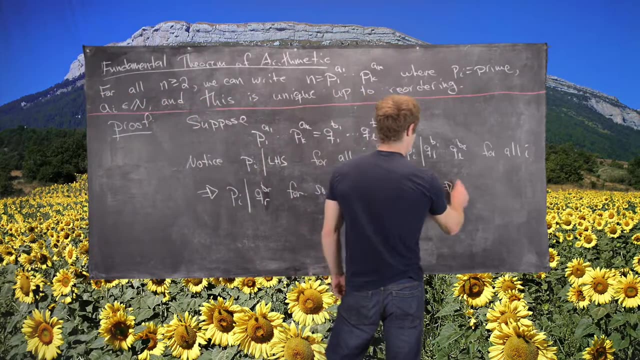 Good, But it follows that that means that P I divides Q, Q R. Good, But then if one prime divides the other, that means they have to be the same. In other words, P I equals Q R. 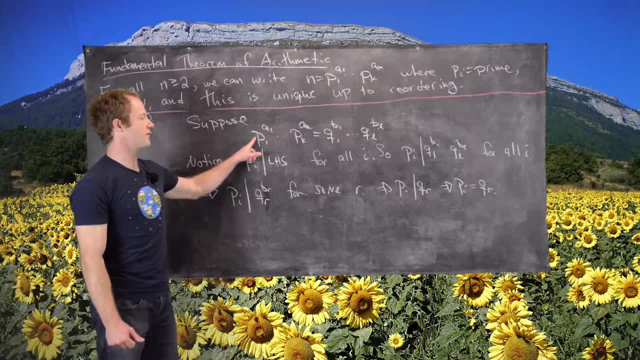 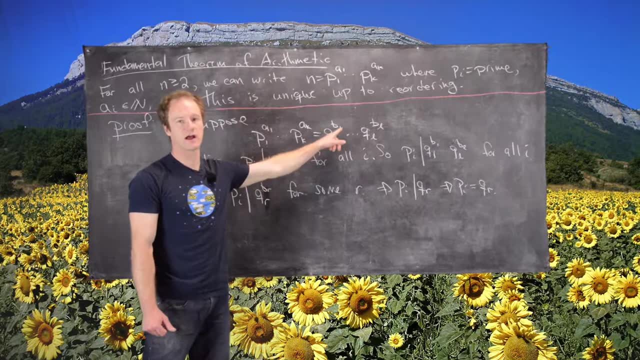 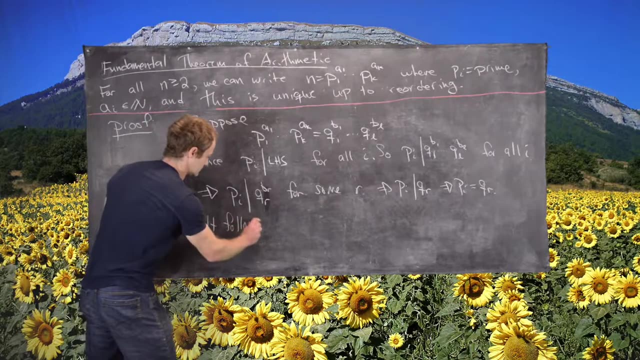 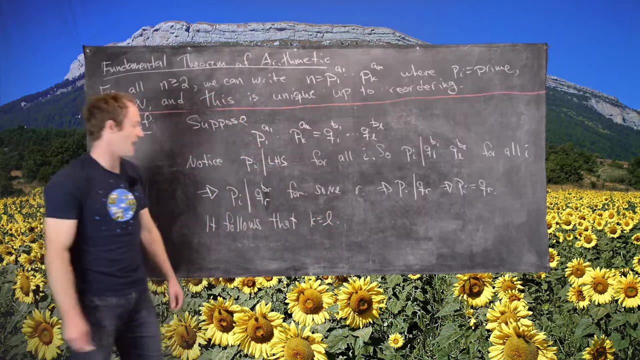 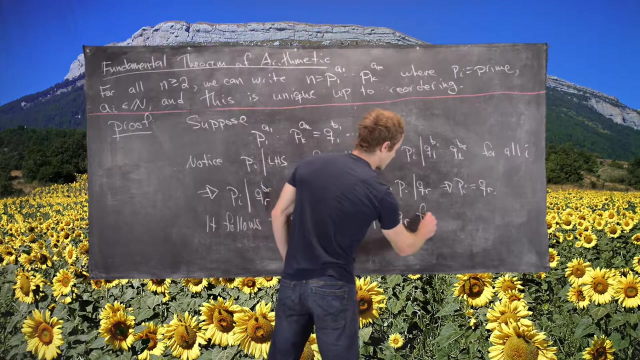 Okay, good. So that means every prime over here is one of the primes over here, And likewise, by a similar argument, every prime over here, every one of these Q's is one of these P's. So it follows that K equals L and P, I equals Q, R for some R. 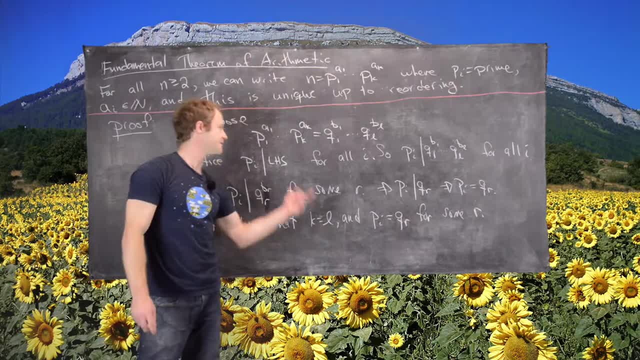 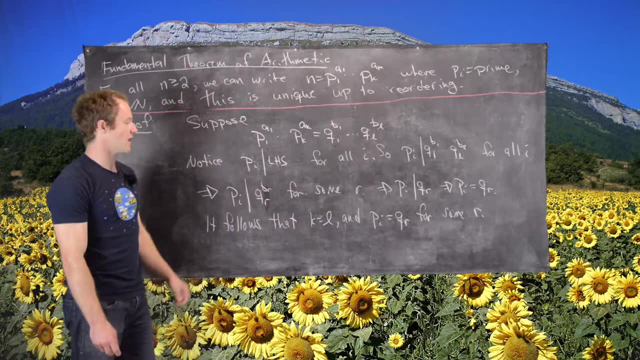 Good. So in other words, not only do we have the same length of primes here, but we have the same primes, So we have the same primes exhibited. So I'll clean up the board and then we'll get on to the next step. 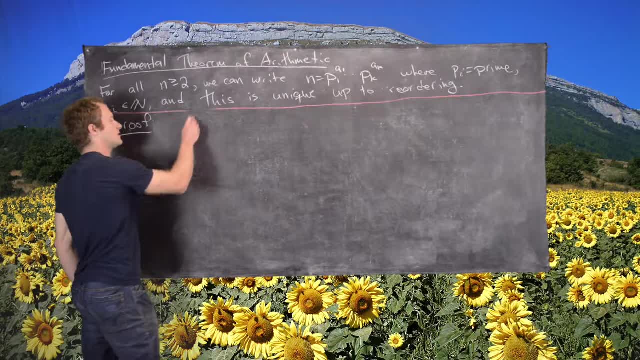 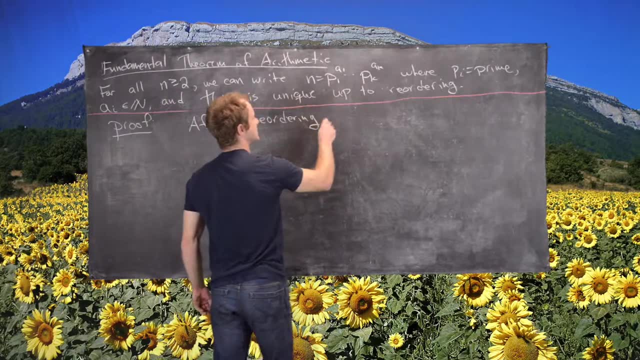 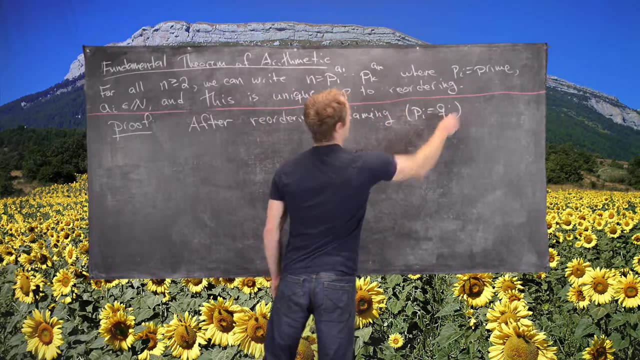 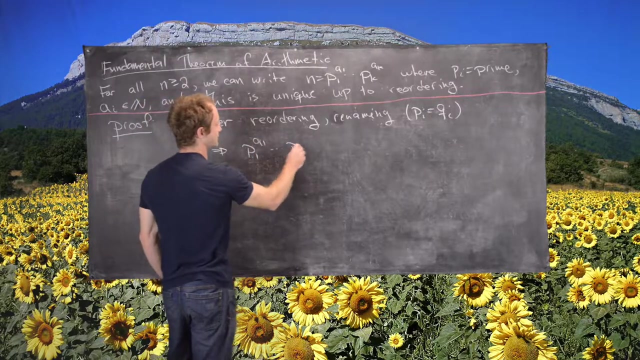 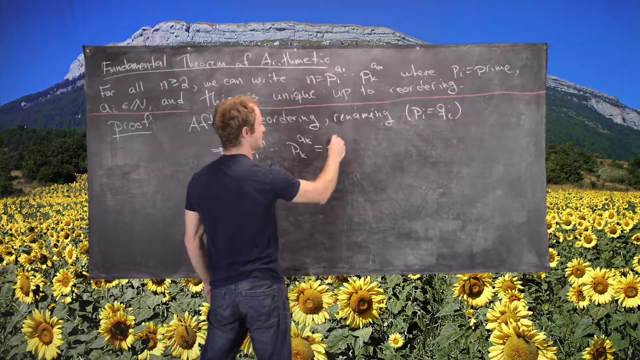 Okay, good, So now, after some reordering, so let's write that down. So after some reordering and renaming, we can set P I equal to Q I, And that tells us the following: P I to the A I up to P K to the A K equals Q I. sorry, equals P I to the B I up to P K to the B K. 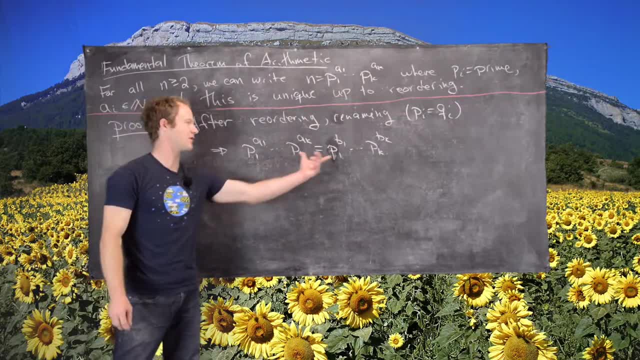 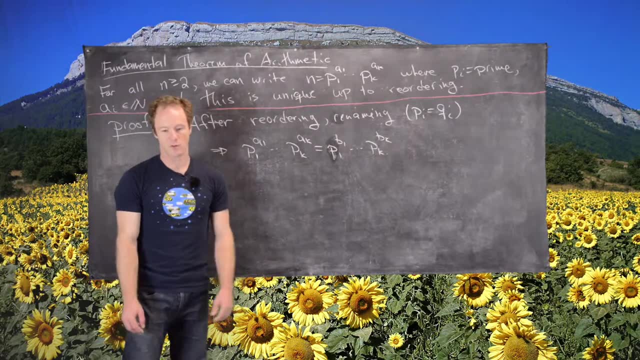 So recall that previously we showed that there was the same number of primes on either side of the equation and they were the same primes, And so we've reordered them so they're in the same order. The primes are in the same order. 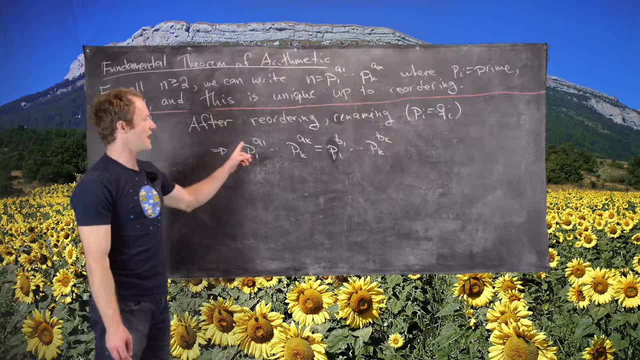 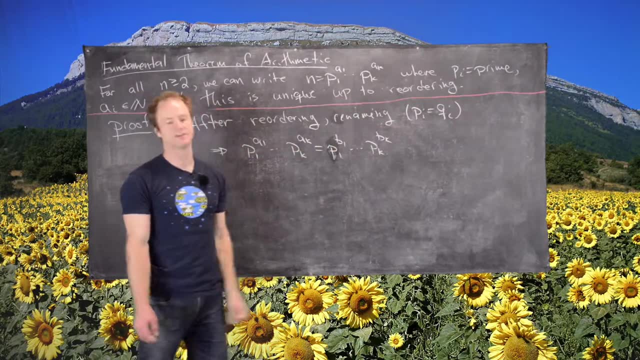 Okay, good, So now we have two cases. Either all of these are the same, so either A1 equals B1, A2 equals B2, all the way up to AK equals BK, in which case we're done. 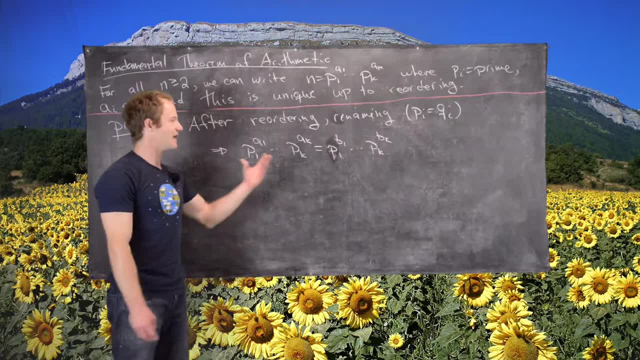 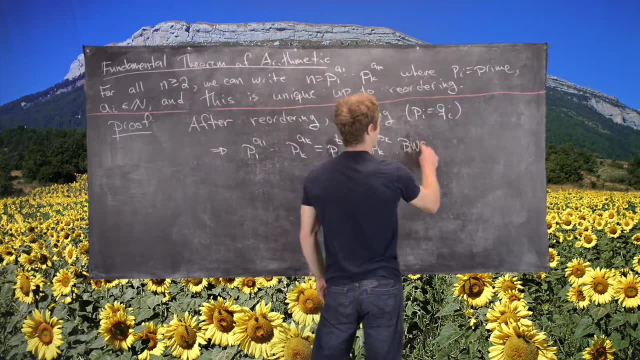 or there's one that's different. So, by way of contradiction, let's suppose that one of these is different, So let's do that. So, by way of contradiction, suppose that A- I is not equal to B I. 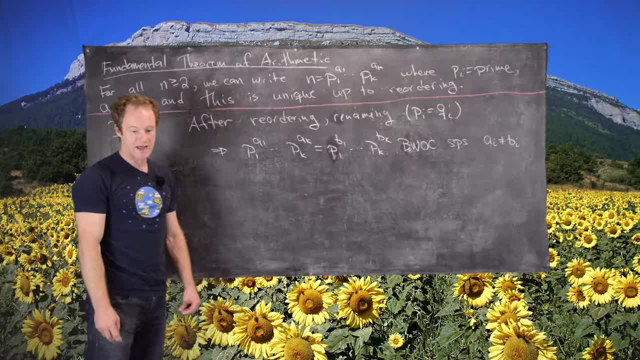 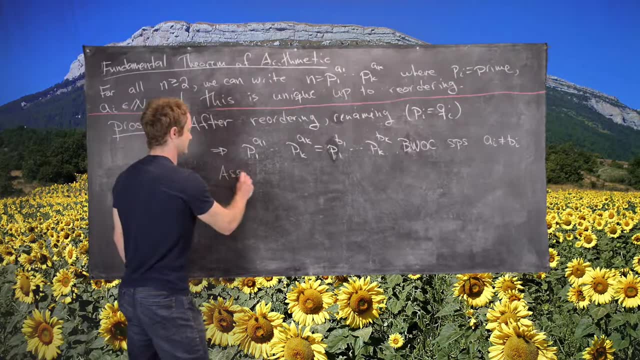 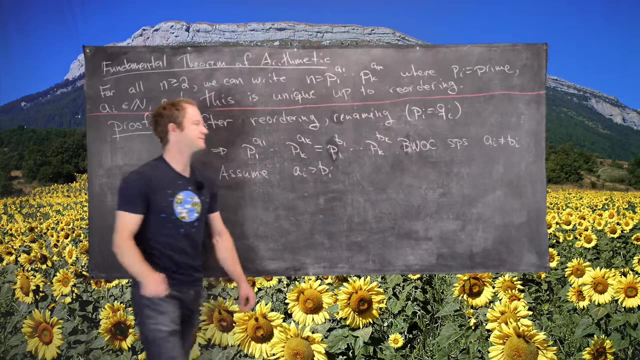 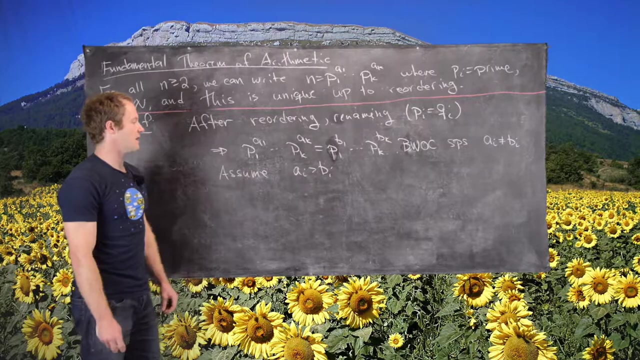 Okay, good, And then we might as well assume that A I is bigger, So also assume that A I is bigger than B I. Good, And now what we'll do is divide each side of the equation. 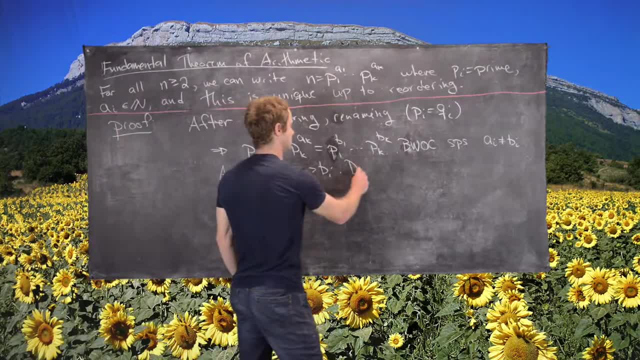 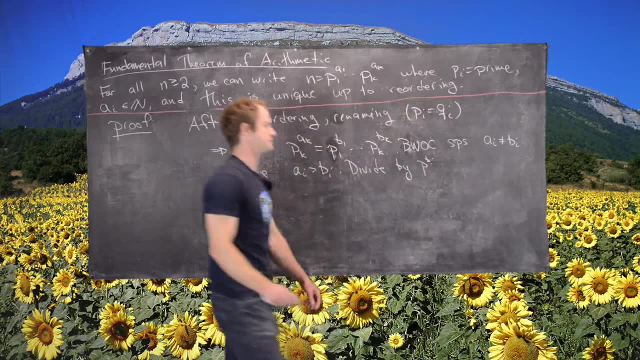 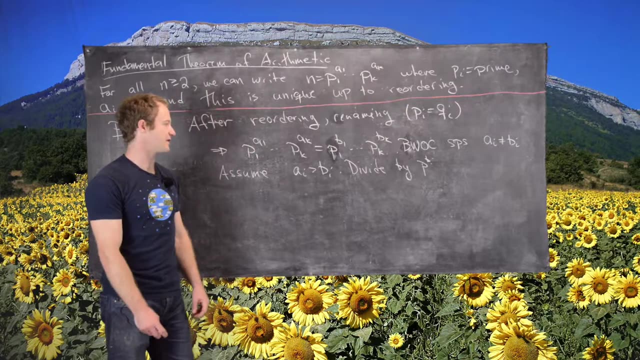 by the following: So divide by P to the B I. Good, So now P to the B I obviously divides the right-hand side of the equation. And then, since AI is bigger than B? I, it obviously divides the left-hand side of the equation. 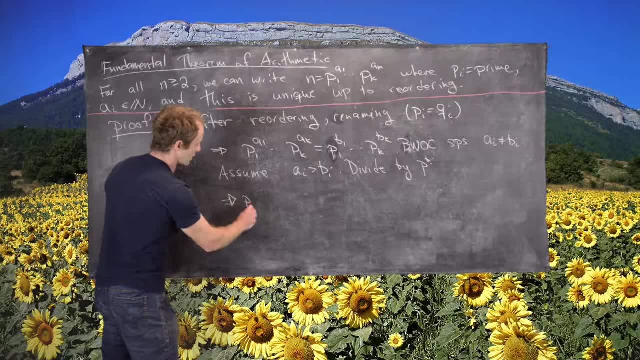 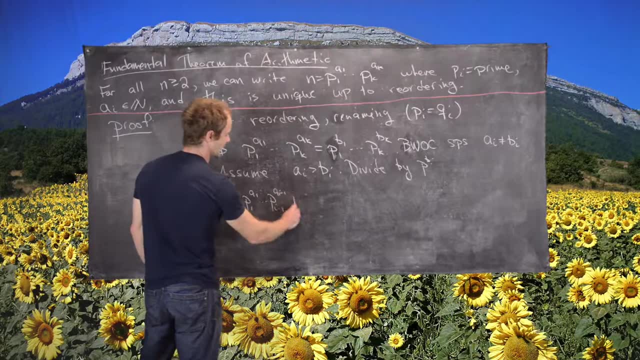 So notice what do we get there? So we're going to get P1 to the A1, all the way up to P I minus 1, to the A I minus 1.. And then we'll have P? I to the A I minus B I.